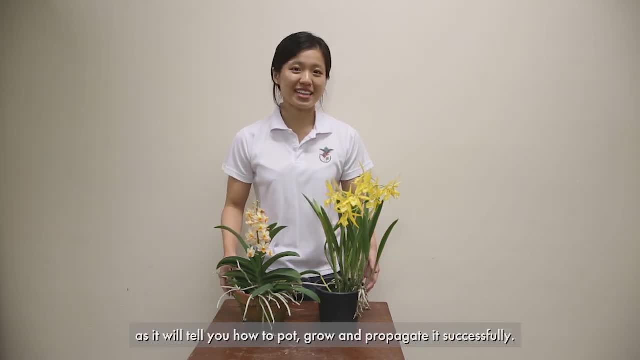 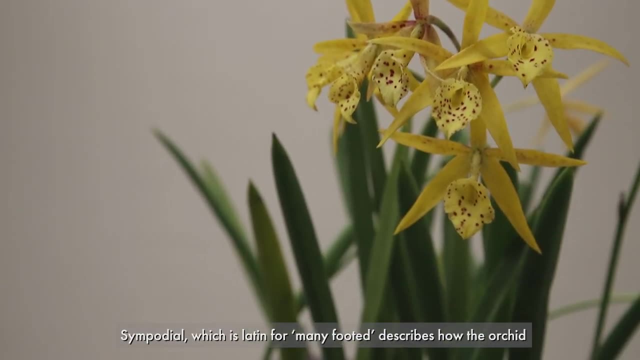 and sympodial. Knowing an orchid's growth form is important, as it will tell you how to pot, grow and propagate it successfully. Sympodial, which is Latin for many-footed, describes how the orchid spreads by putting out new shoots from the horizontal stem at 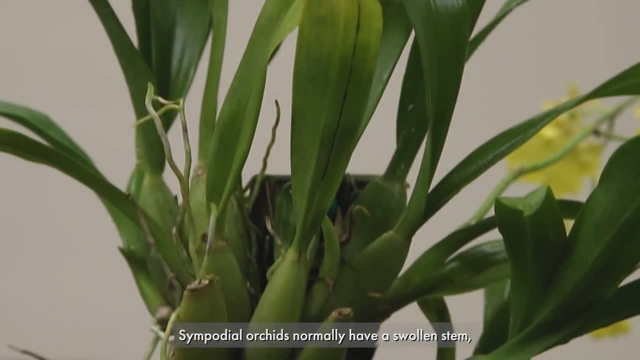 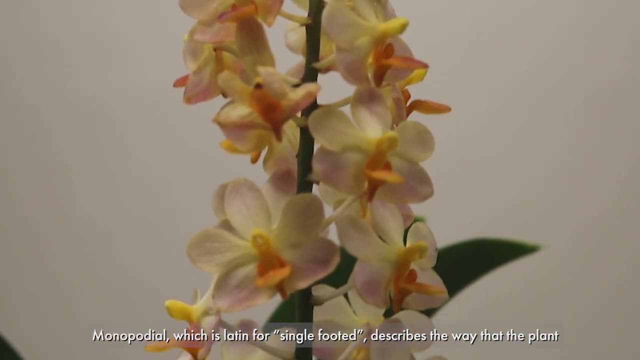 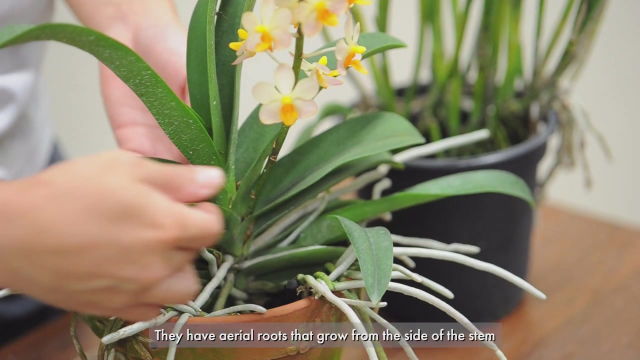 the base of the plant. Sympodial orchids normally have a swollen stem, known as a pseudobulb, which stores water. Propodial, which is Latin for single-footed, describes the way that the plant grows. from the top of the plant, It puts out new leaves at the top. They have aerial roots that grow. 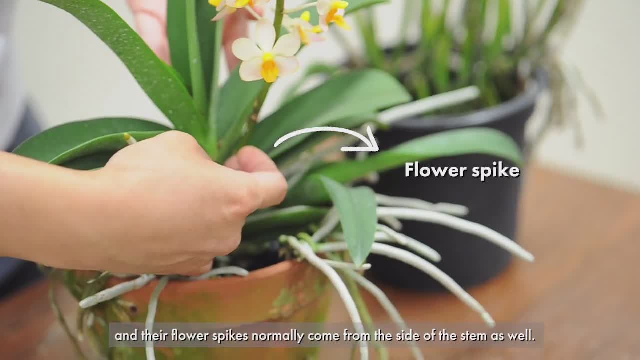 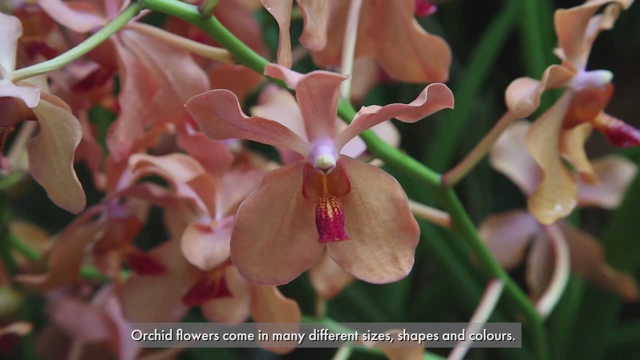 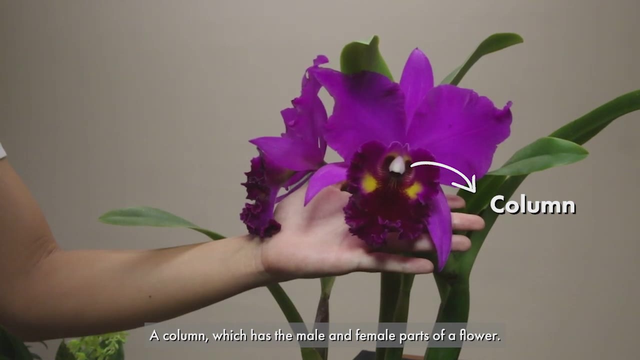 from the side of the stem and their flower spikes normally come from the side of the stem as well. Organ flowers come in many different sizes, shapes and colours. The organ flower consists of a pedicel, a column which has the male and female parts of a flower, three sepals. 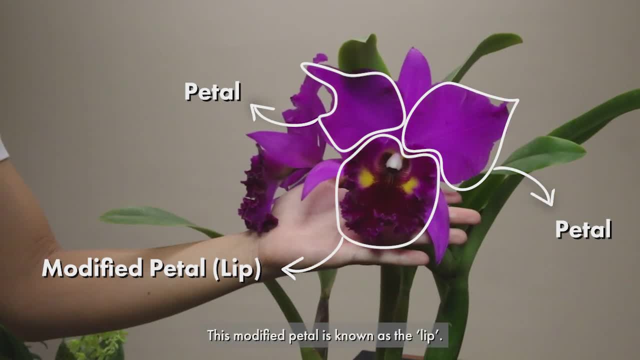 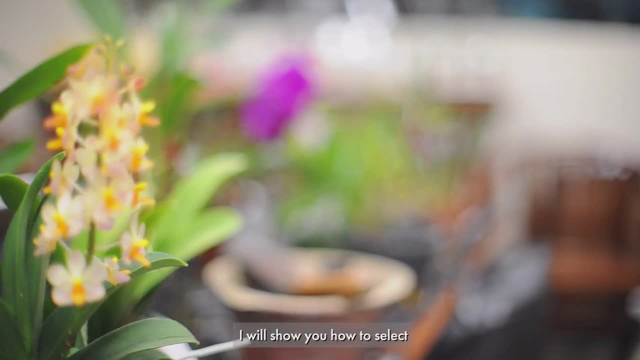 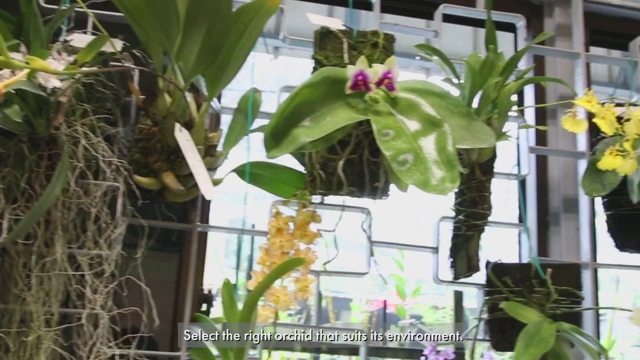 and three petals. One petal usually stands out. This modified petal is known as the lip. Now that we've covered the basics, I will show you how to select a good quality orchid suitable for growing indoors. Select the right orchid that suits its environment. It is always easier to take care of a plant. 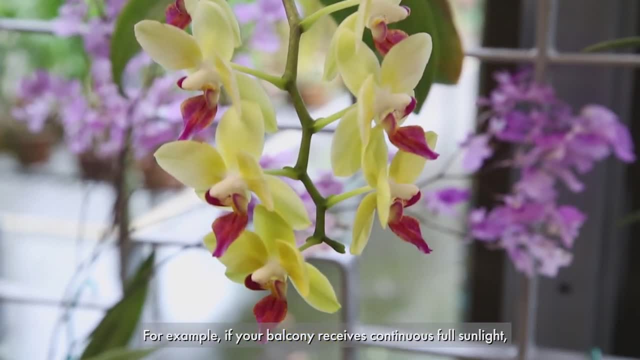 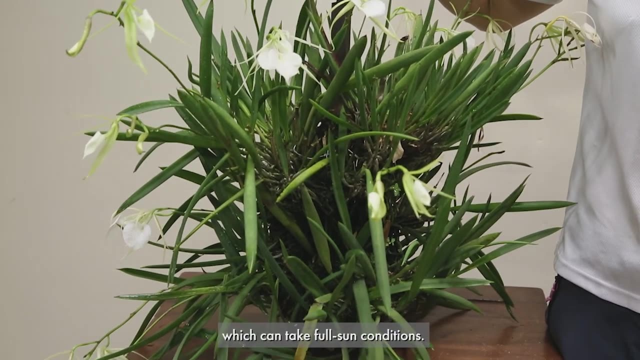 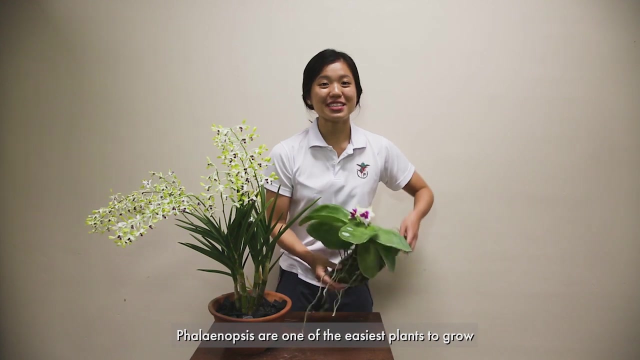 if you provide it with the right conditions to grow. For example, if your balcony receives continuous full sunlight, buy an orchid such as the Brassavola lady of the year. Two orchids which are commonly grown at home are Dendrobiums and Phalaenopsis. Phalaenopsis. are one of the easiest plants to grow and bloom several times a year. Dendrobiums are generally hardy and have pseudobulbs which are able to store water. To select a good plant, check these four things: Good quality flowers that are not deformed, healthy and 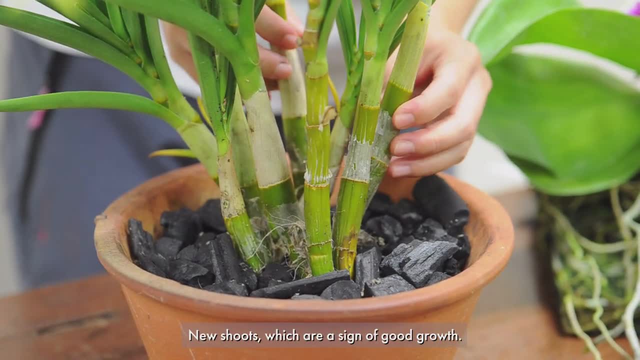 succulent pseudobulbs with healthy leaves, new shoots, which are a sign of good growth, healthy roots with good growth and healthy leaves that are not deformed. You can also buy roots with green tips and roots that are not rotting. 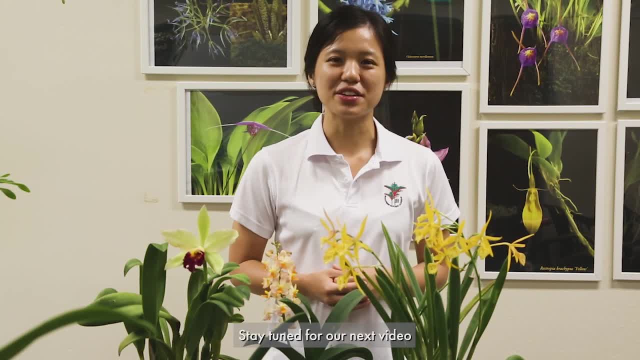 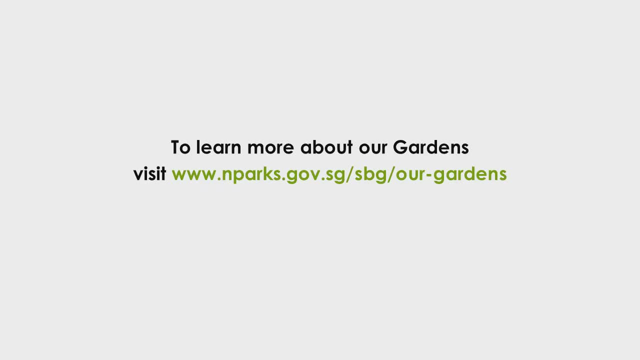 Now you know a little bit more about orchids. Stay tuned for our next video, as our orchid expert will be sharing with us how to take care of orchids. We'll see you next time.